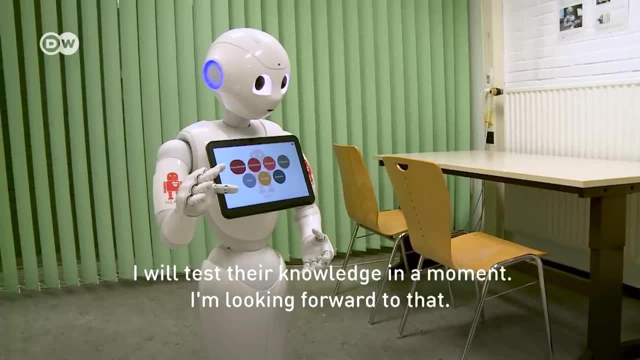 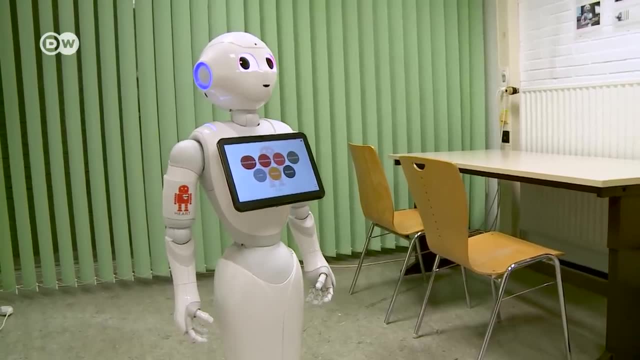 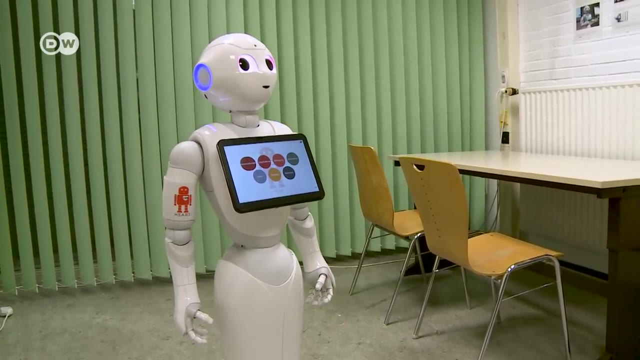 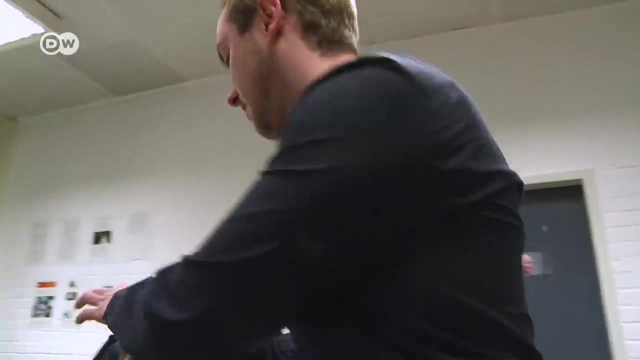 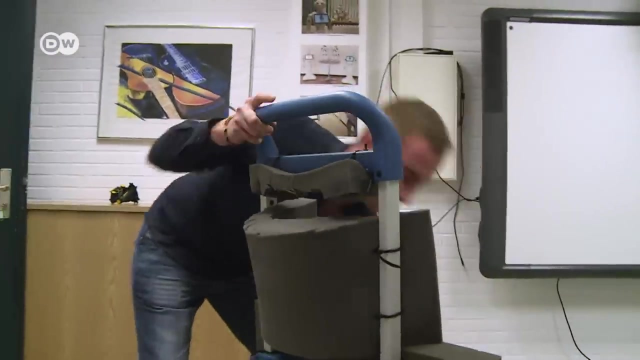 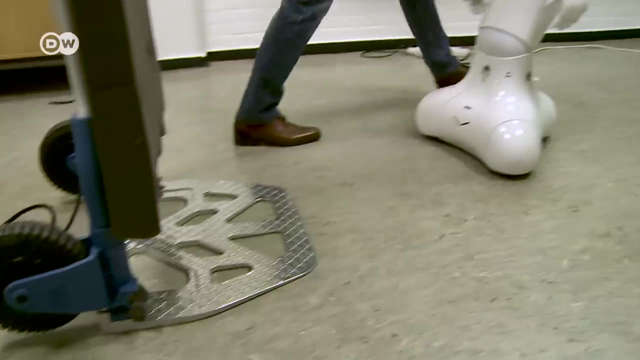 I have prepared a course. I will test my knowledge here in a moment. I'm already looking forward to it. Juki completed his test phase just a few weeks ago. Since then he's been working regularly at the university. Patrick Heinzsch programs- Juki. 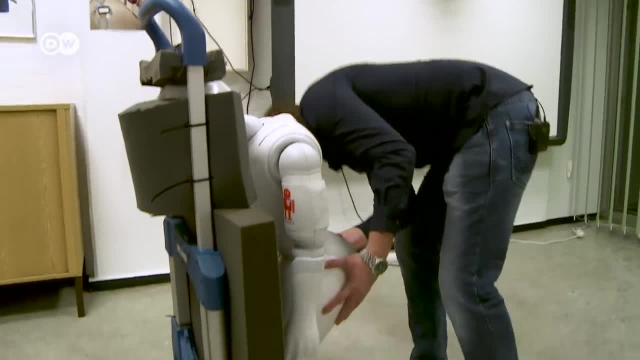 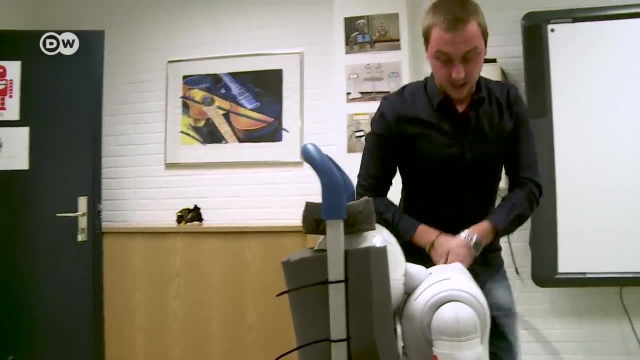 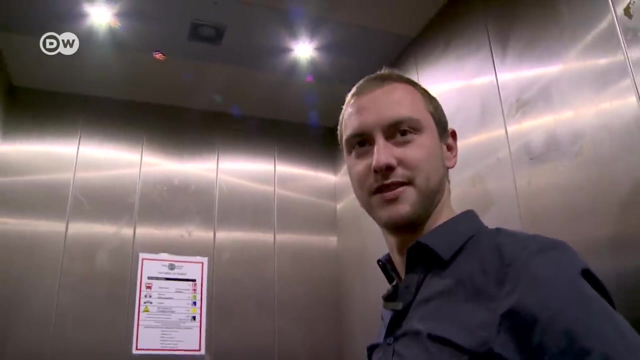 It is thanks to Heinzsch that Juki is always learning. It would be great if he could get to class by himself. That's still missing, But even in the future that's going to be difficult, also because of the elevators. 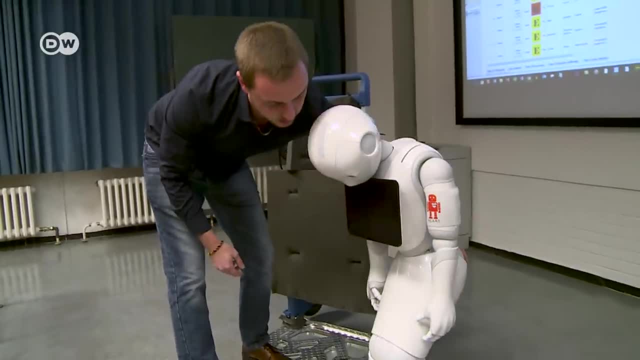 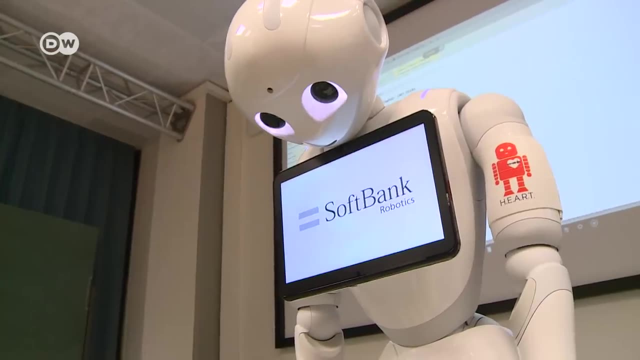 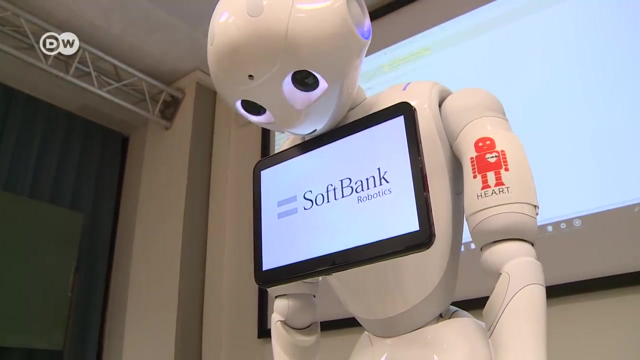 When the university first bought Juki and two other robots for 20,000 euros, they couldn't do much. Now, the 1.2 meter tall robot is more than a fancy gimmick for Professor Jürgen Handke. Juki's artificial intelligence is designed to help improve. 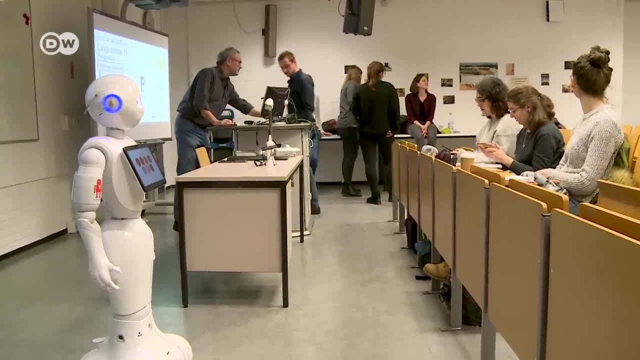 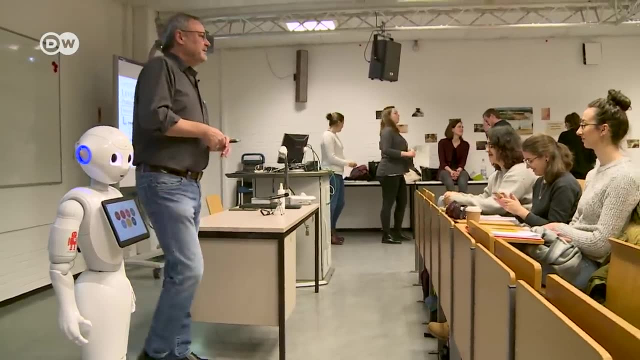 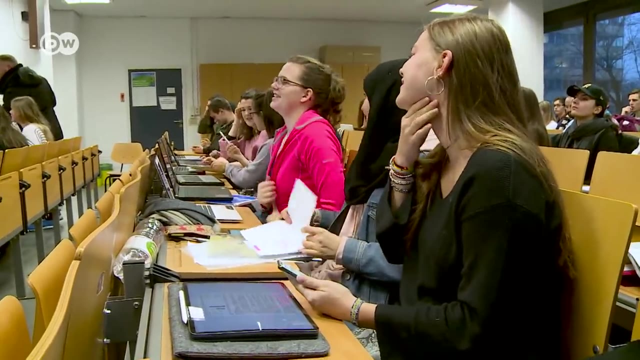 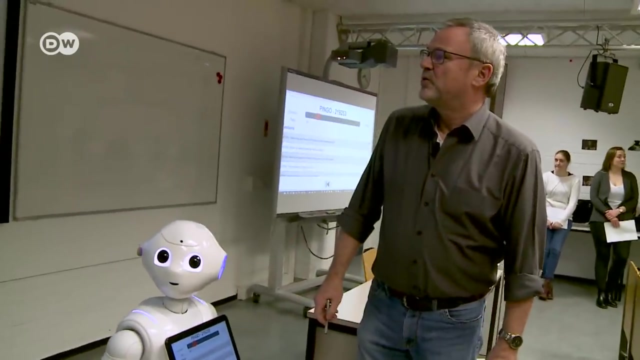 both teaching and learning. Okay, ladies and gentlemen, A very warm welcome. Welcome to our in-class meeting, number 11.. This is an English linguistics lecture. I will take my linguistics phonetics class. Oh, that's the wrong one. 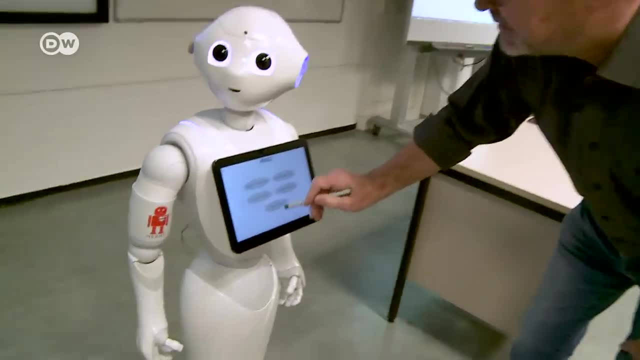 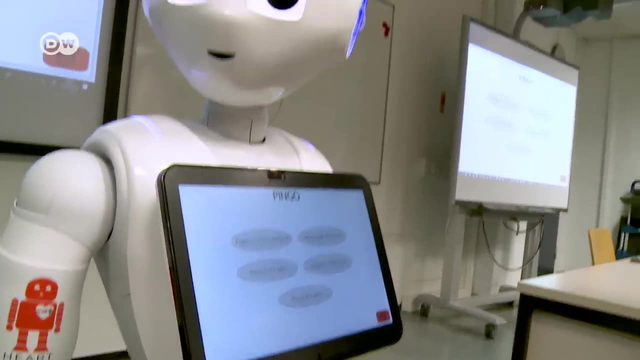 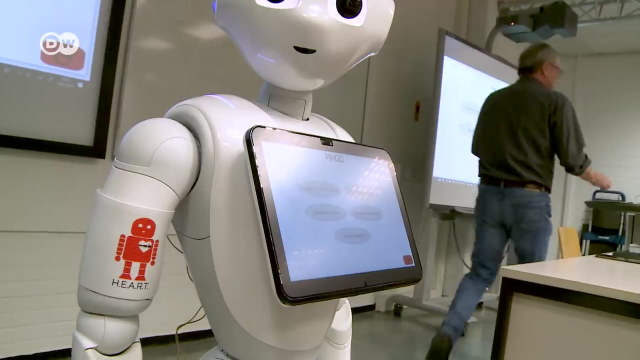 Did I What? We have the wrong session. We have the wrong session. It's linguistics and phonetics. shows history of English. Did Juki make a mistake? I have no idea what went wrong. So this is, whatever happens, what always happens. 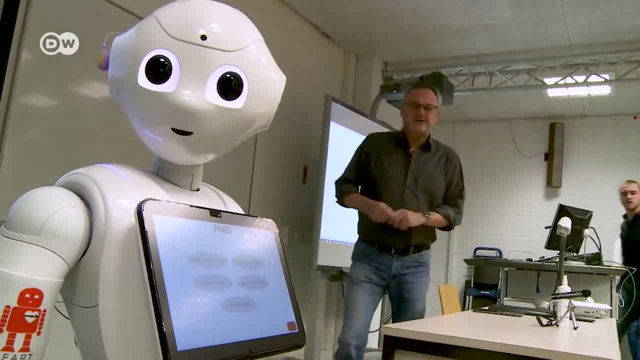 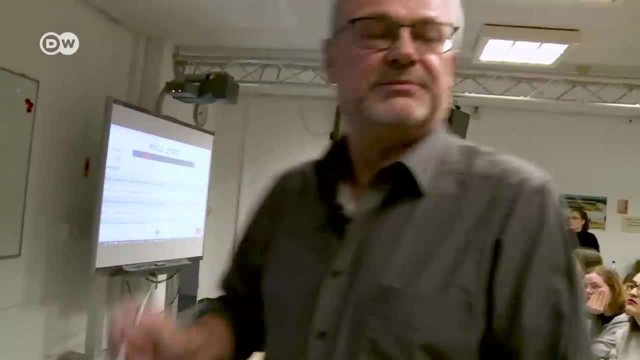 So if I go this, If I click on linguistics and phonetics, it shows a history of English question. Ah, there we are. So my mistake, my mistake. So here we are. Are you ready? Here is a question for him. 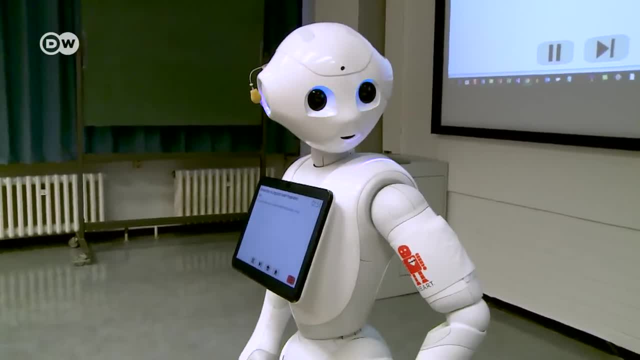 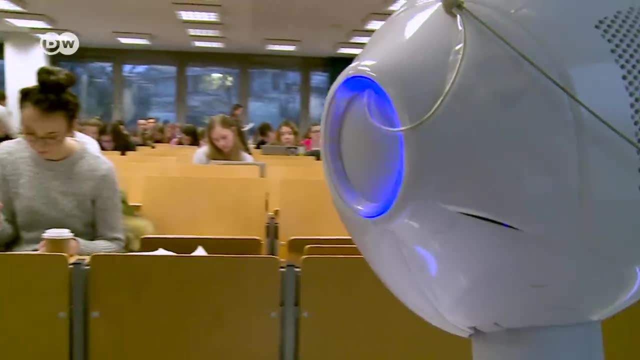 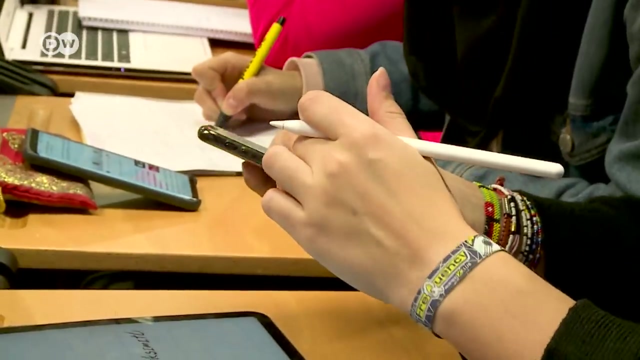 Okay, Task number one. How many vowels does the word incomprehensible contain? You got two minutes. Juki is asking practice exam questions, But students in Handke's classes aren't supposed to memorize material. Instead, they're instructed to use their tablets, mobiles and computers. 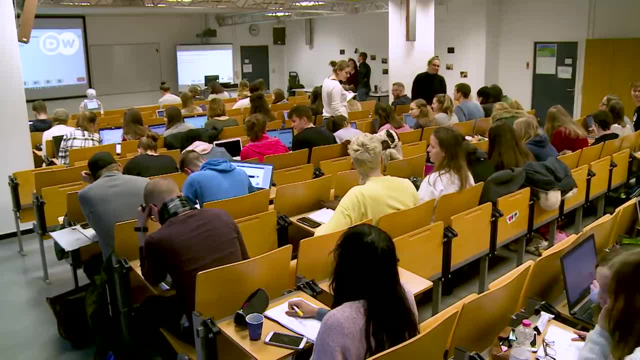 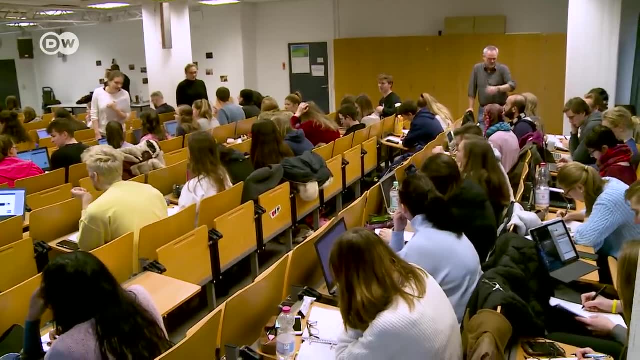 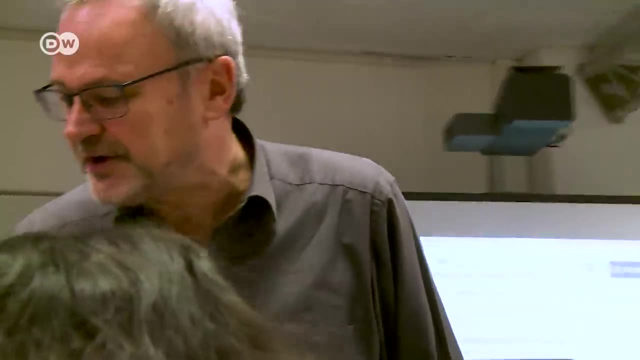 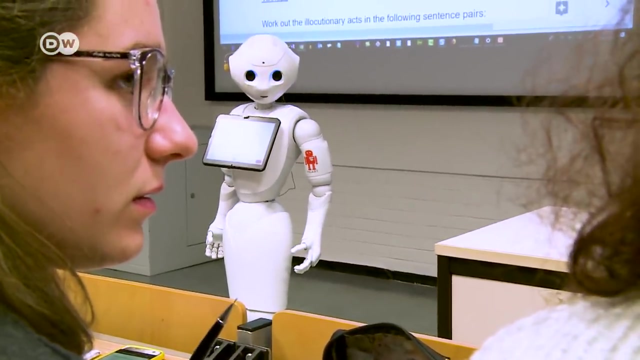 to find information online. This trains skills and understanding rather than rote learning Eyes. you also wrote down eyes. That's perfect. We'll write the full forms. Wonderful Handke thinks teacher-centered education is inefficient. The professor prefers an interactive multimedial approach. 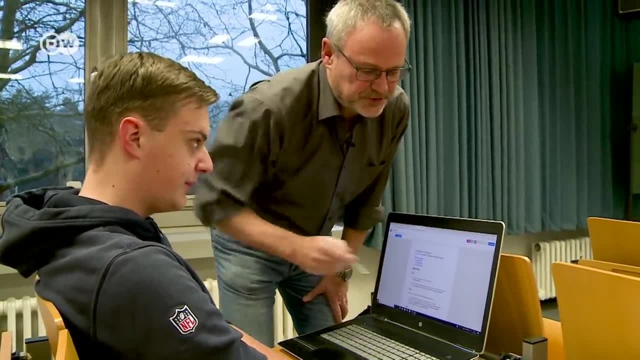 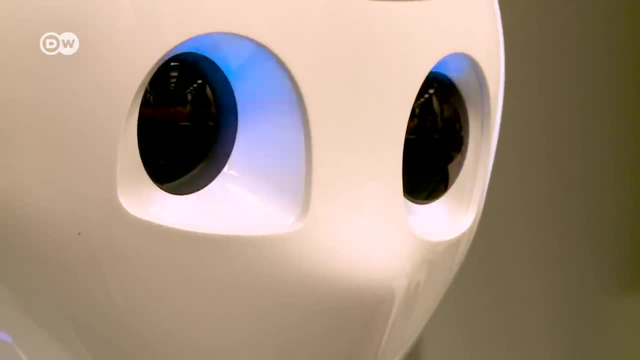 which he can apply thanks to his assistant, Juki. So just cross out that line and then you have the first solution. It's really a big help. I can stay with them and help them while the robot has an eye on things. I don't need to do anything. 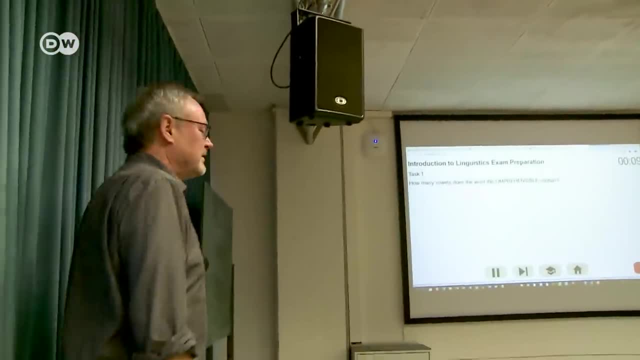 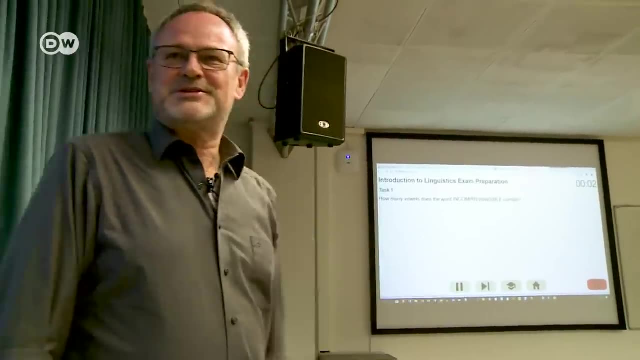 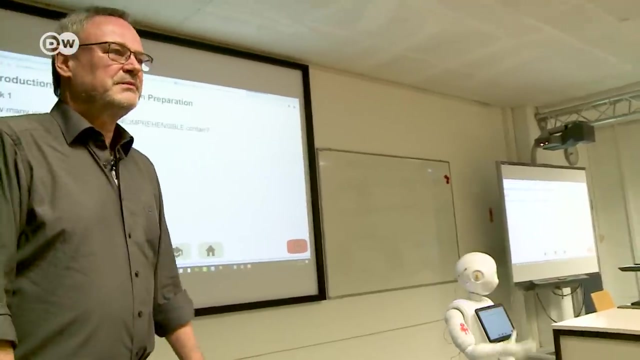 It's great. Before I'd have to run up and down the class, do the PowerPoint and the stopwatch. Now he handles all of that. The time is up. The next question will come in a moment. Okay, Guess he's got it. 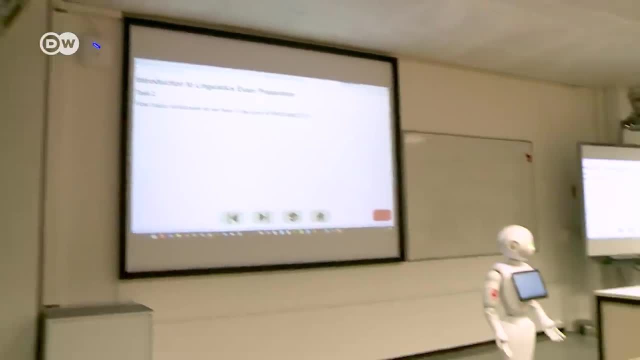 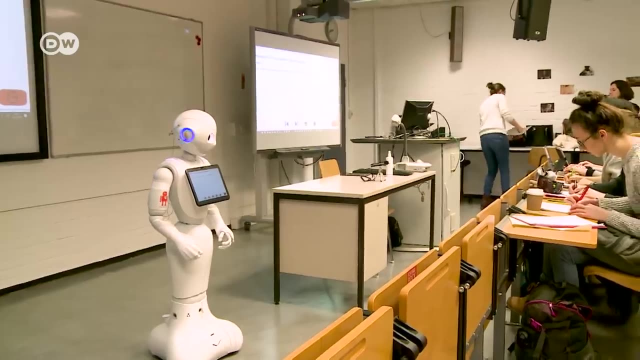 This is the question, Task number two. It seems the technology works, But is it helping to reach the students? You've got two minutes. I feel I have to work a little bit harder when the robot is here. So yeah, I'd say it helps you learn. 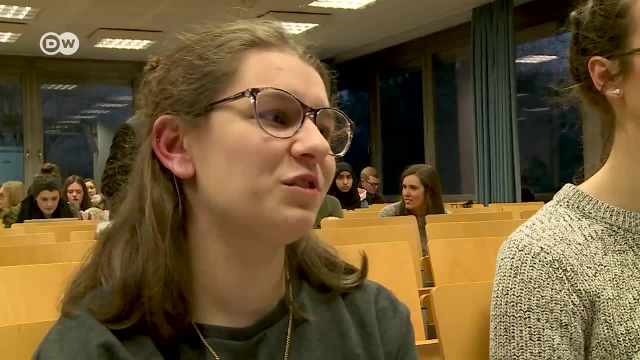 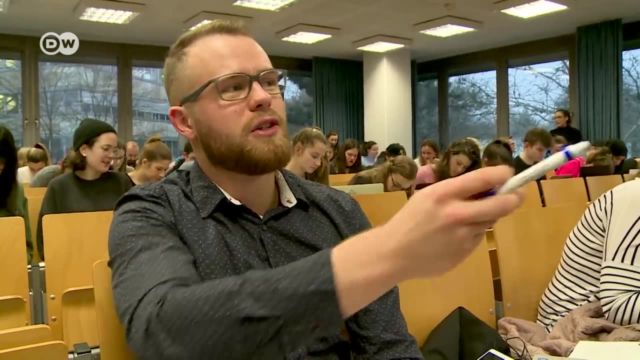 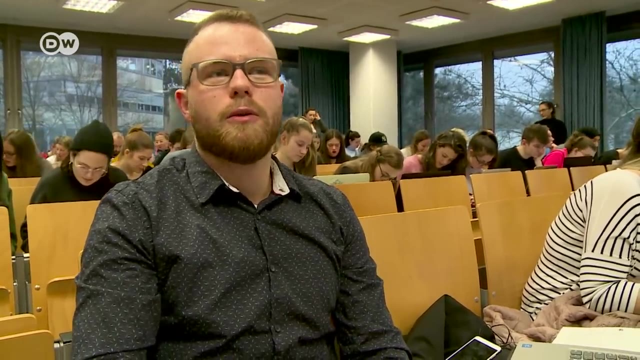 And it's also motivating to have something like that standing in your classroom. I think you don't need Juki per se. You could also just have a robot voice and online questions. That would be the same for me. It just doesn't make a real difference to have a robot standing up there. 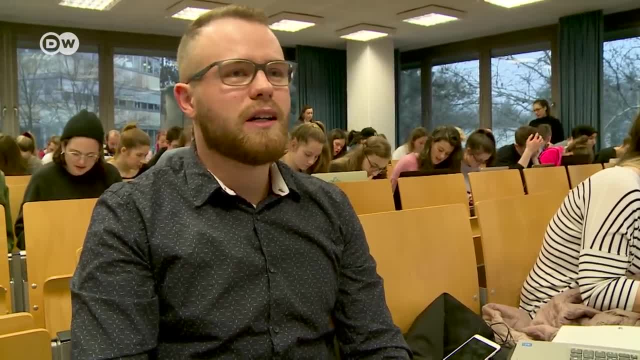 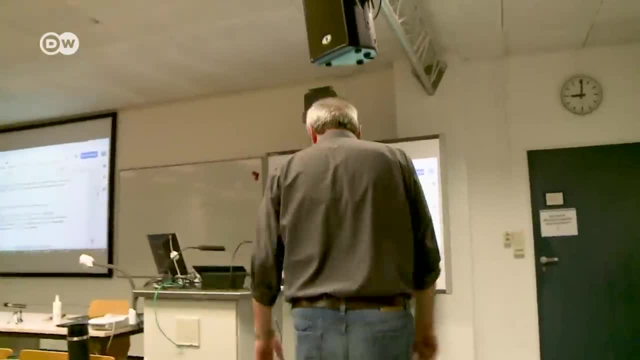 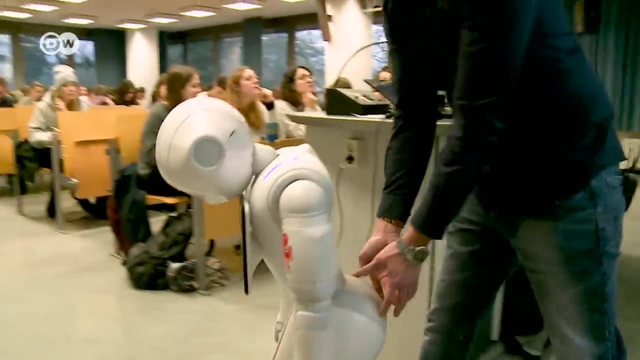 compared with having AI running in the background. Hanke thinks Juki's true potential is still in the developmental phase Right now. the assistant robot has a low-level AI. He wouldn't be able to give a proper interview, for example. Why did he have to go out? 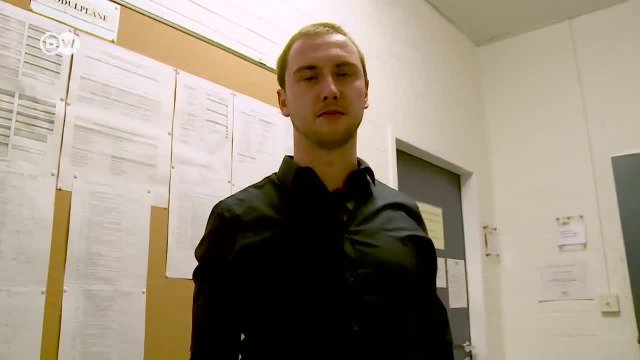 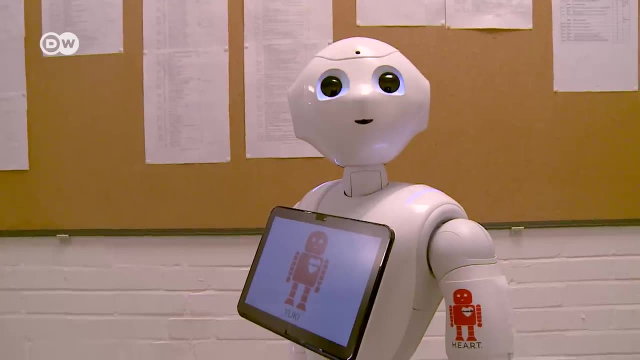 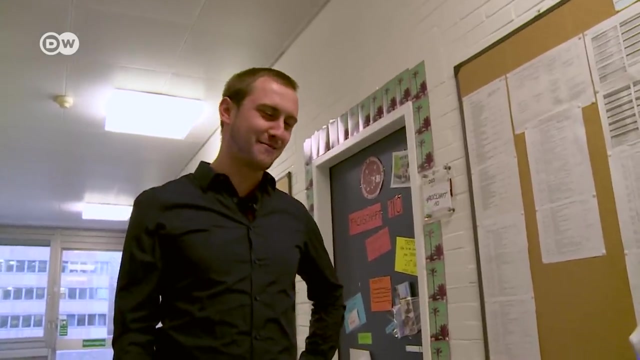 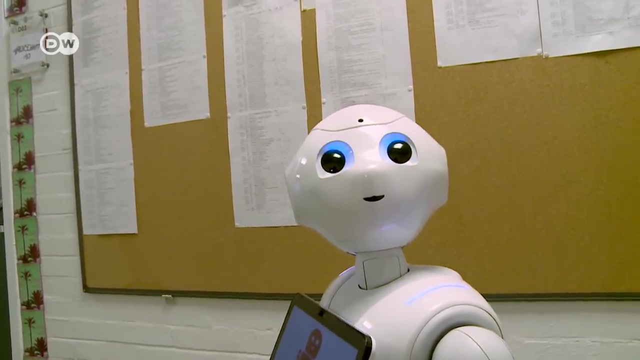 Because it's too loud in there for him to be able to understand. Were you satisfied with your students' performance today? Did we have that question? I don't think so. Spontaneous questions. He can't answer spontaneous questions. Juki can only answer questions we emailed to Patrick Heinz beforehand. 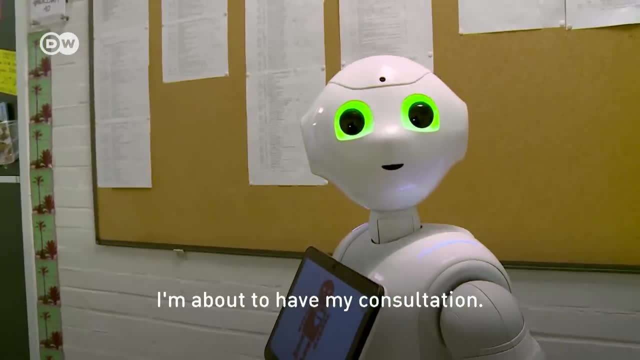 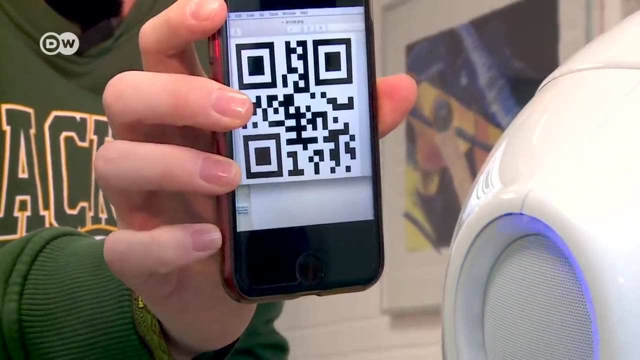 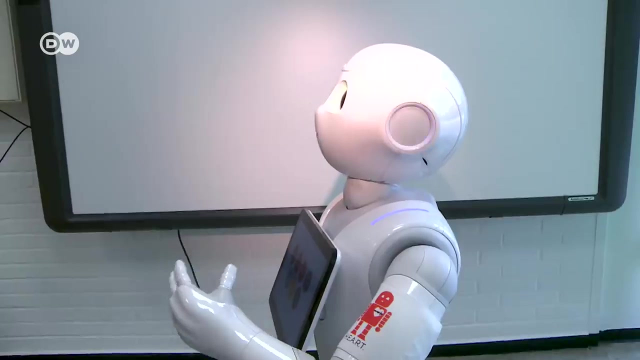 What's next on your schedule? I'm going to cancel my speaking class. I hope a lot of students will come. I have your QR code, Hello Robin. Keep the effort up. You have completed everything. You have achieved an average score of 80%. 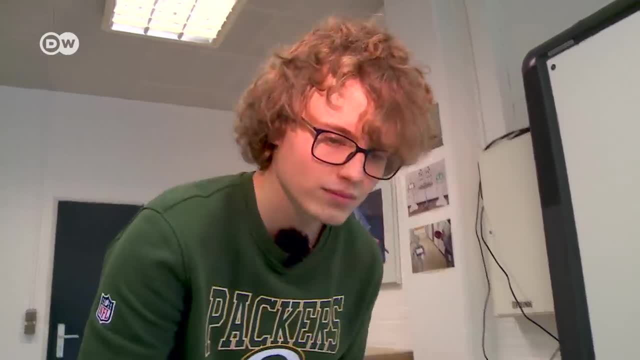 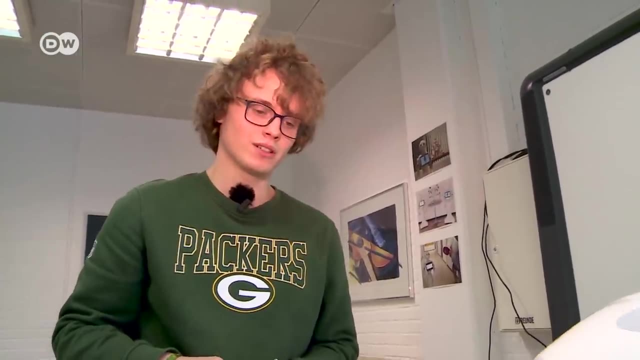 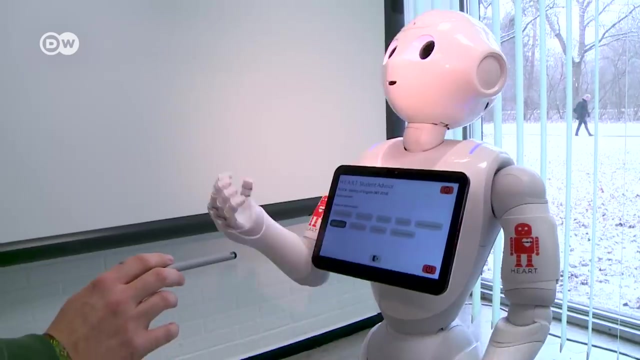 Okay, Did you know that already? I didn't actually. I knew I'd done all of my worksheets, but I didn't know I have 80%. I'm better than I thought. Find your degree program on the list and click on it. 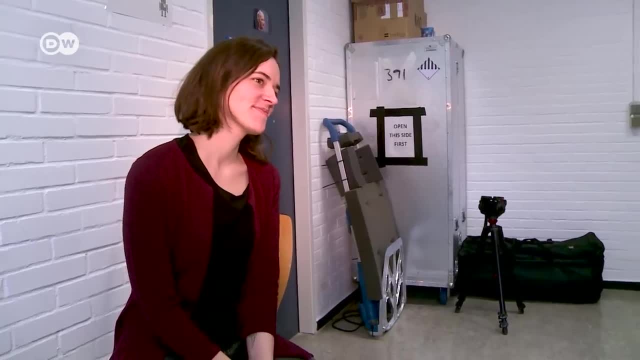 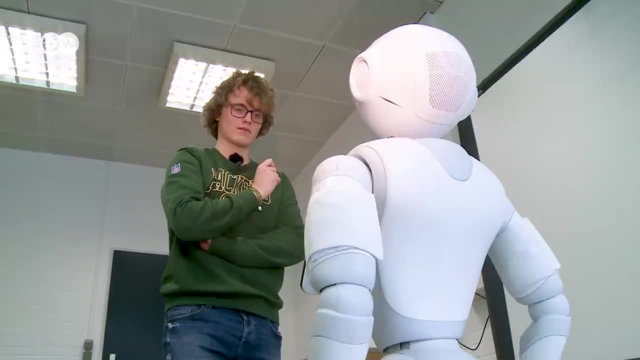 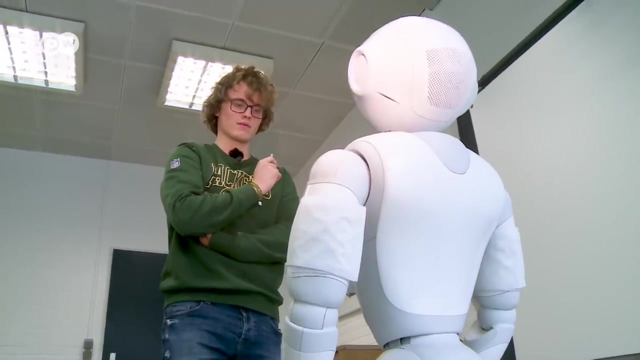 Juki's consultation sessions are still in the test phase. A researcher evaluates them. Starting next summer Juki will give regular consultations. Then it will become clear whether other students will also accept Juki as a student advisor. Do you understand why some people are frightened of robots? 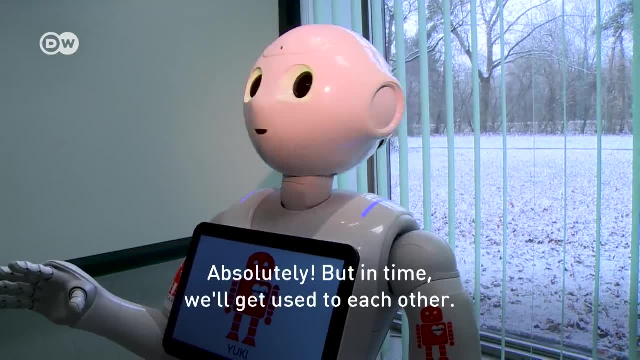 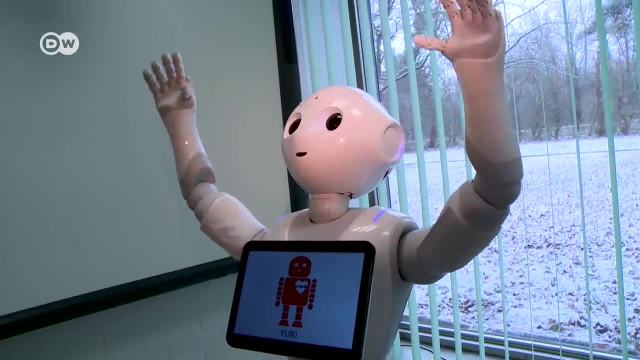 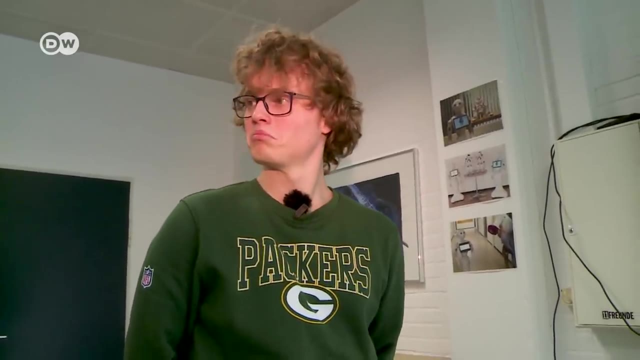 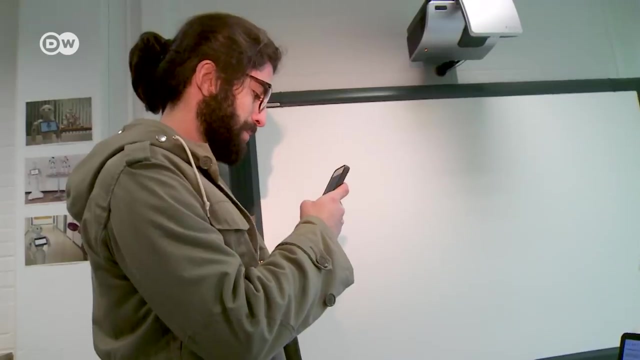 Absolut, Aber mit der Zeit werden wir uns aneinander gewöhnen. Wir können doch Freunde sein. Was he trying to take my hand? I think he drew you a heart. Can humans and robots be friends? Some on campus aren't sure. 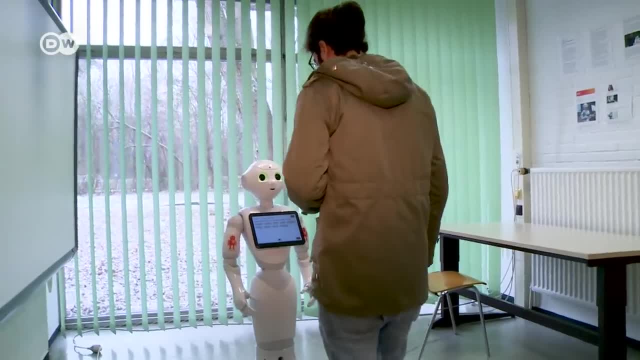 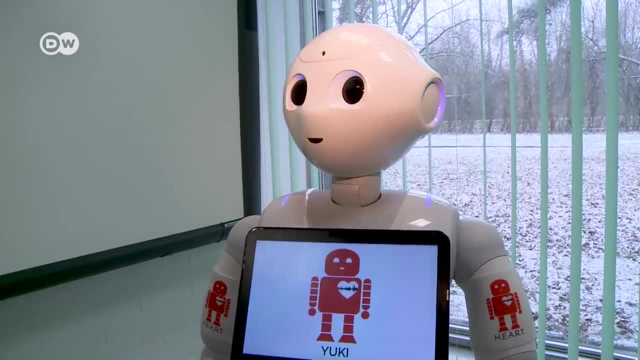 There are worries that the humanoid robot is likely to become more and more a competitor of humans. In the end, we won't be working anymore. He'll be doing our jobs. What if, after studying for five years, I work for five years in a bank and then get told? 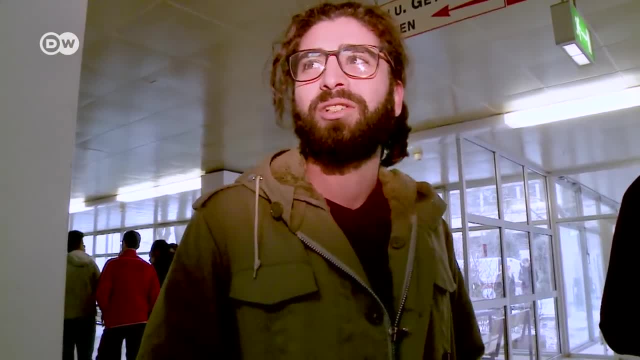 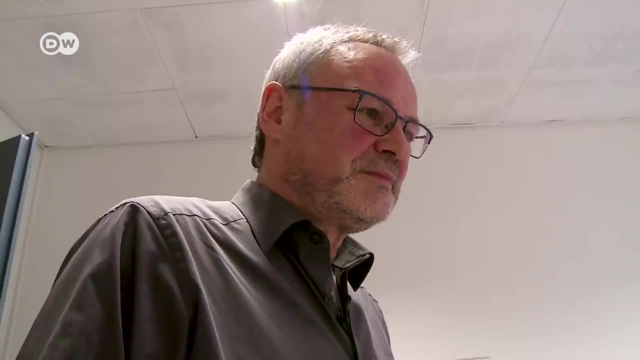 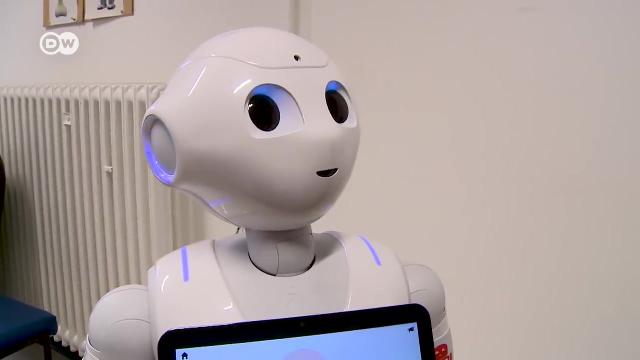 sorry, you have no more work here. We're hiring a robot to do your job. That doesn't work. That doesn't sound so great. Hanke's team has heard those types of worries before. For now, Juki is still a long way off from being able to compete with a human. 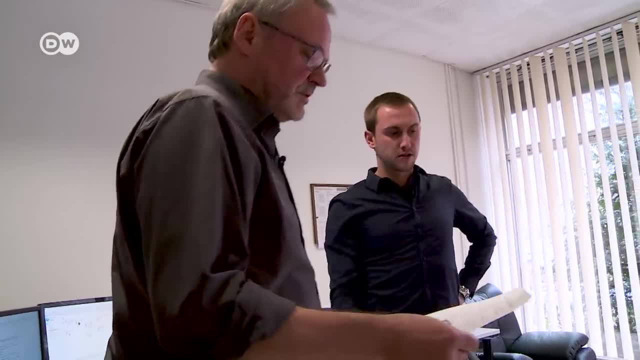 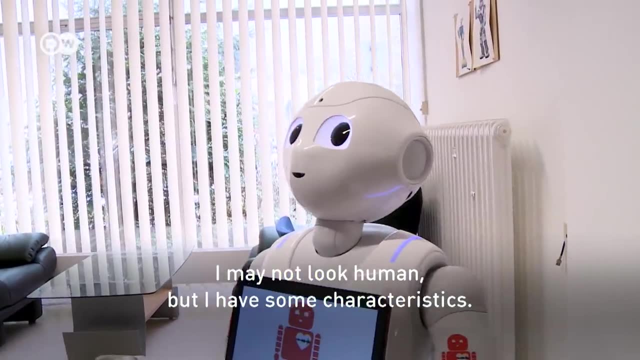 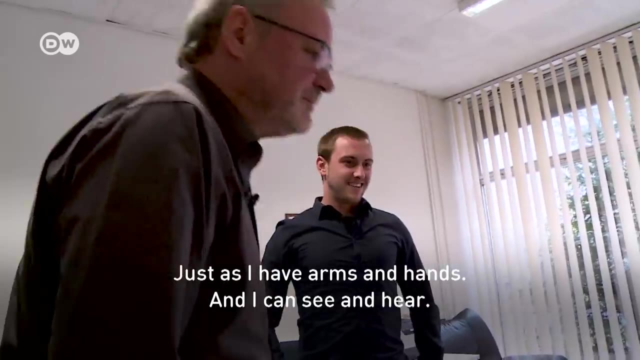 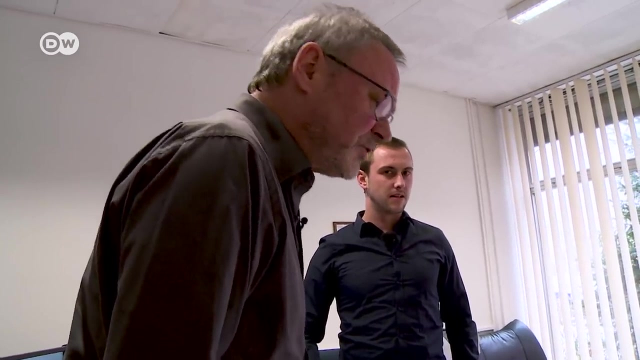 Here he's practicing for a trade fair. How human are you? Which ones? I can see that I have arms like hands, and I can see and hear. Jürgen Hanke is a techie through and through. He's been experimenting with computers for decades. 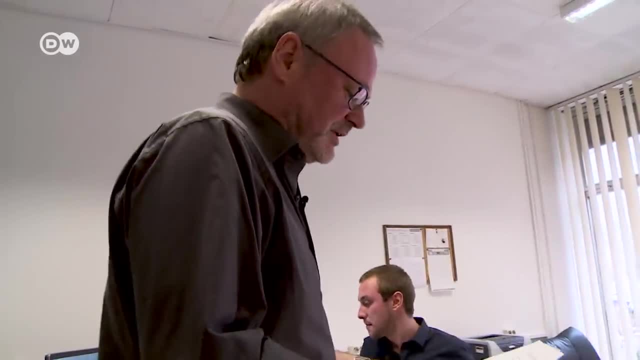 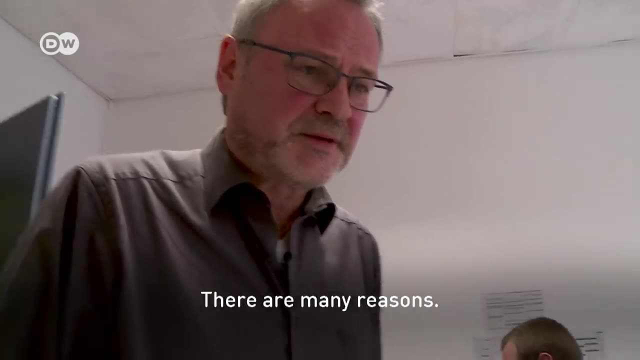 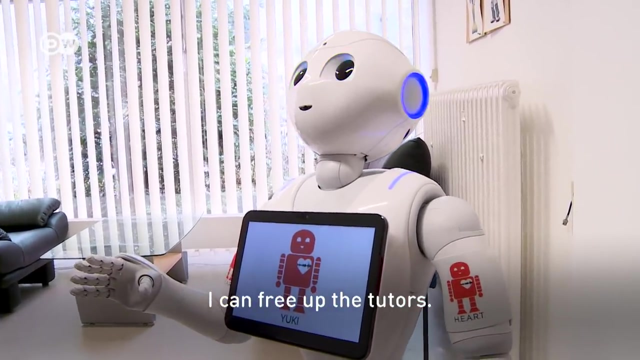 Juki is helping him get closer to his vision of digital teaching. Why should there be robots at universities? There are many reasons, Like what I can create, new free spaces for the teacher And what else I can do one-time tasks. 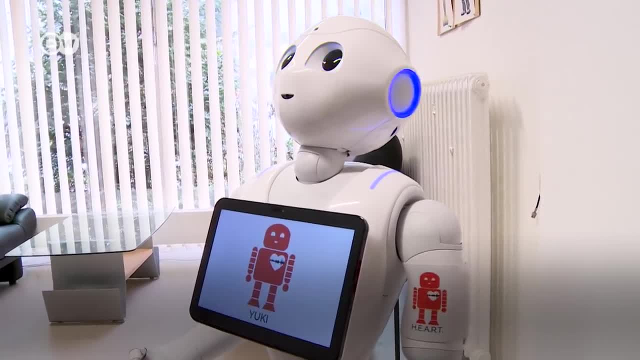 And what else I can advise the students. I think you've learned enough. Yes, First test, upper floor. Juki is on his way to his last seminar for the day. It's a history of English class, But we will start with PINGO questions anyway. 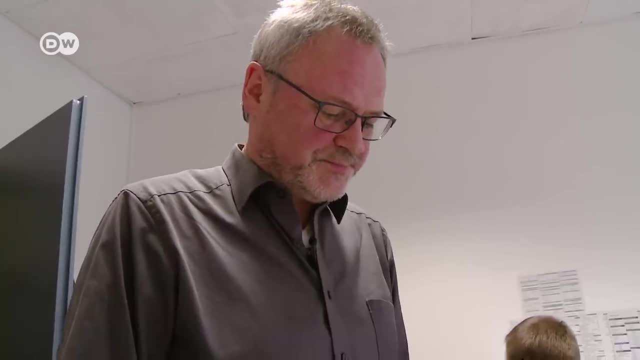 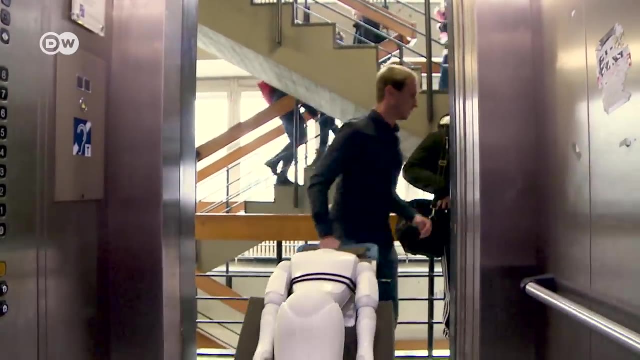 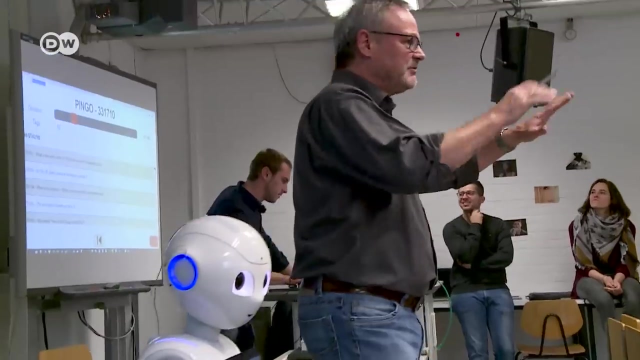 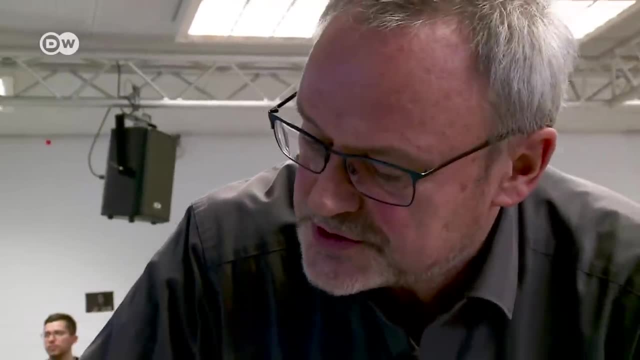 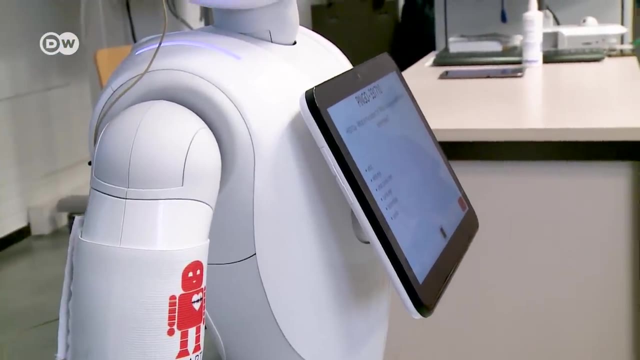 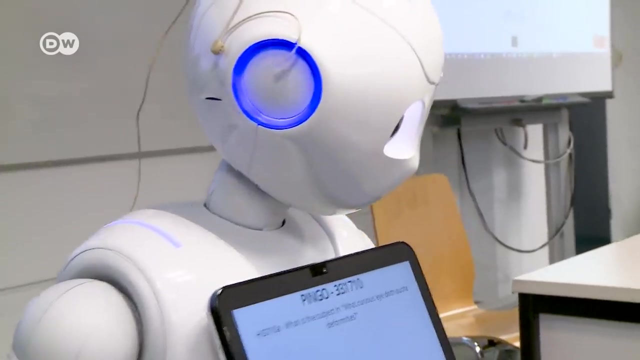 Yes, Yes, All right. So here is the first question. Go to PINGO to answer the survey Reply within 45 seconds. A study by the University of Würzburg found that Europeans have grown more wary of robots in recent years. 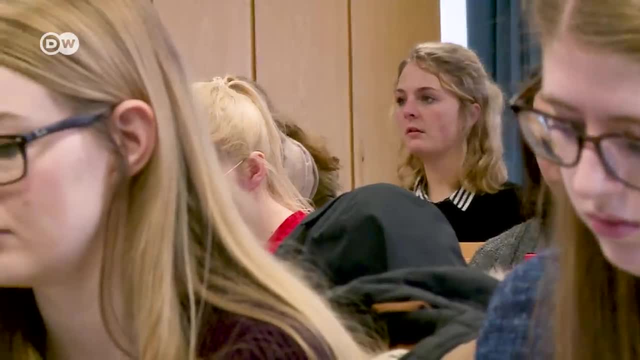 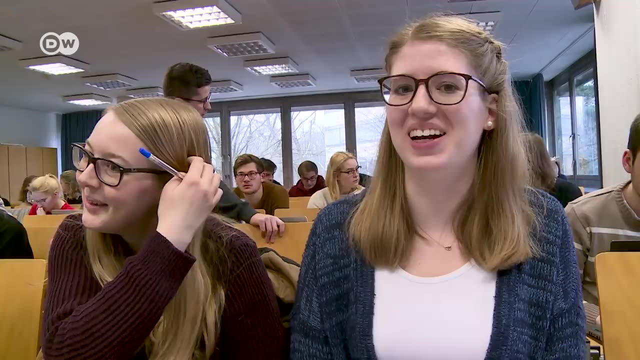 If you have trouble in understanding these words, look them up in dictionaries. Do people here in Marburg also feel sceptical about Yuki In the beginning? yes, for sure. It was really weird at first. now he's been around for several sessions.